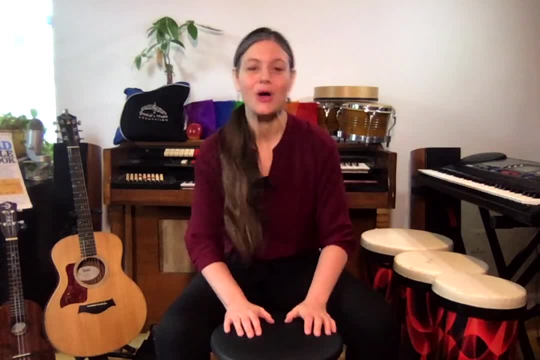 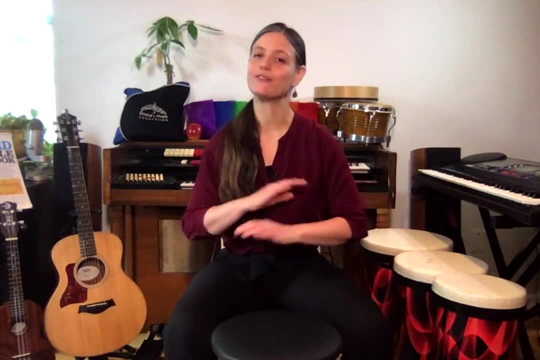 make sure to check out our previous video on makeshift drums. Alright, so to get started, there's two different parts of this song. We'll have the verse and we'll have the chorus. Now the verse: you can play anything that you want. It's musician's. 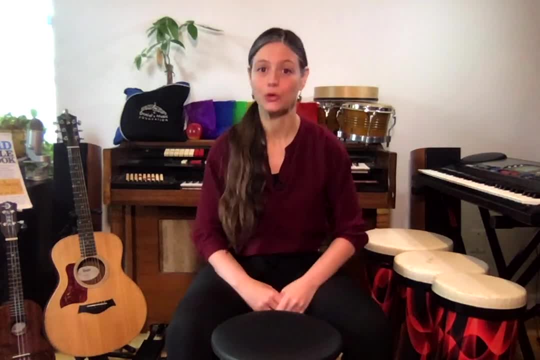 choice. So anything that you hear, anything that you feel, you're welcome to play it. The verse is the part of the song that tells the story. The chorus is the part of the song that repeats For the chorus. we're all going to play the same pattern together, So for 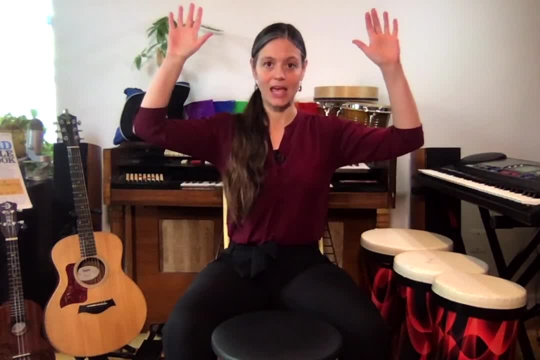 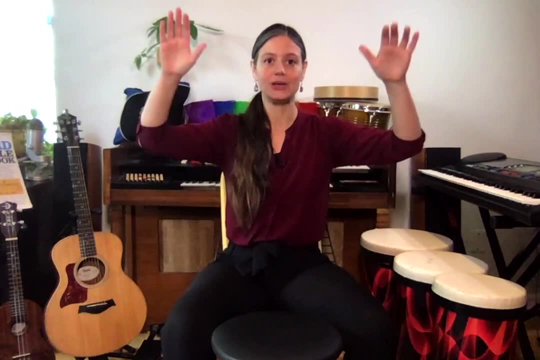 this pattern: you're going to put your hands up in the air and then you're going to bring them down twice. So bang bang and then bring them down, Bring them back up. Bang bang, bring them back up. 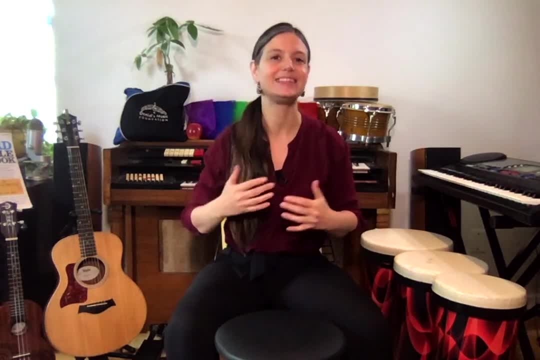 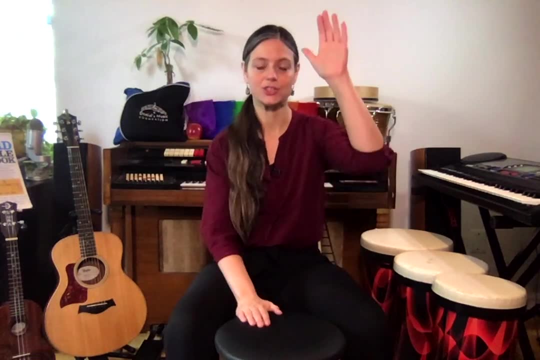 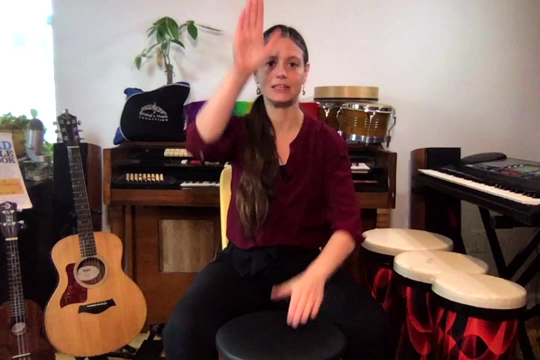 For the next part. what I want you to do is alternate your hands. It doesn't matter if you're using the same hand. I am just as long as you're having a good time, So you'll bring one down and switch. We call that alternating. Okay, And let's take it a little faster. 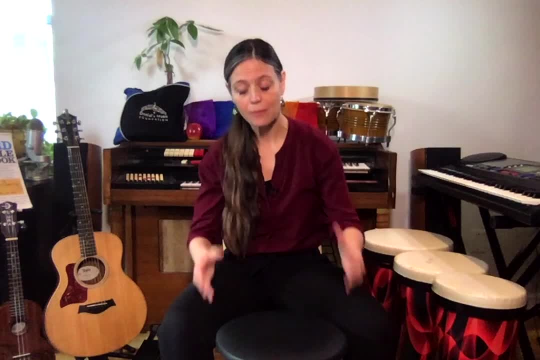 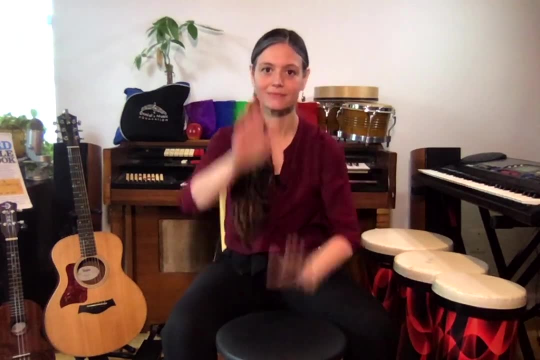 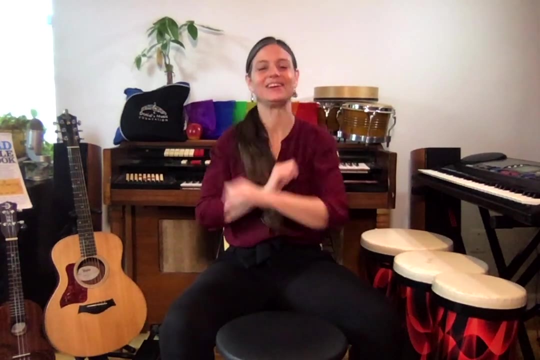 Very nice. So when that part of the song is on, I will refer to that as walking, because it sounds like my hands are walking on the drum. Now let's get a little faster, A little faster, A little faster. Good, When we get super fast, I'm going to call that running. 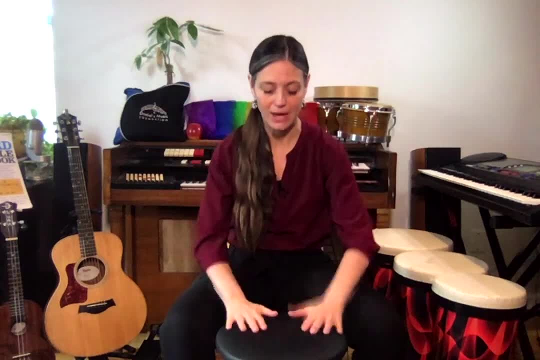 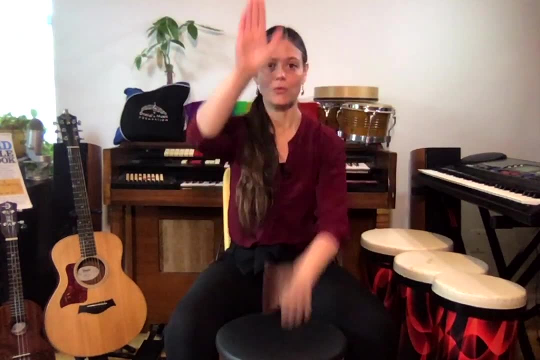 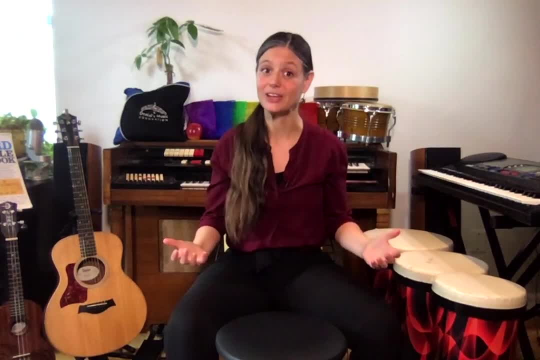 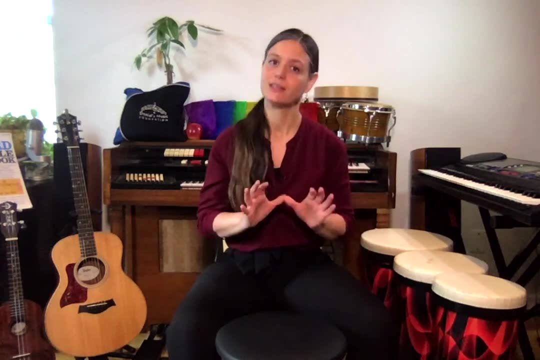 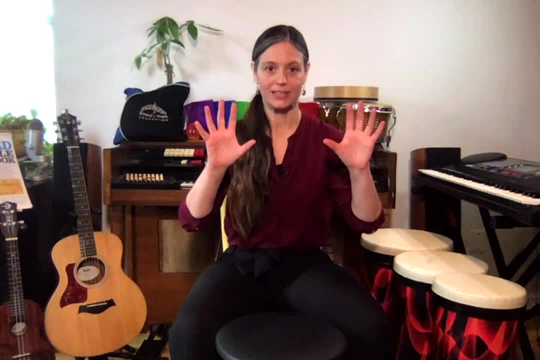 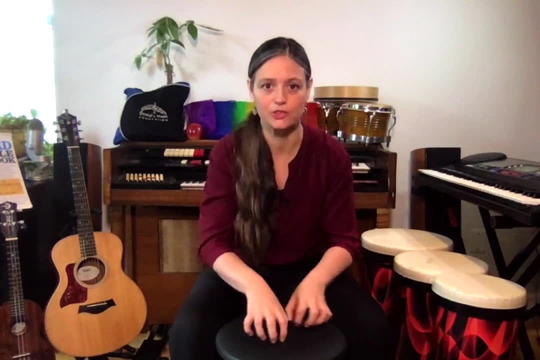 of different things. The first is scratch. So I want you to take your hands and curl your fingers over like a lion, Okay, And you're going to use your nails to scratch on the head of your drum. Now for some people. 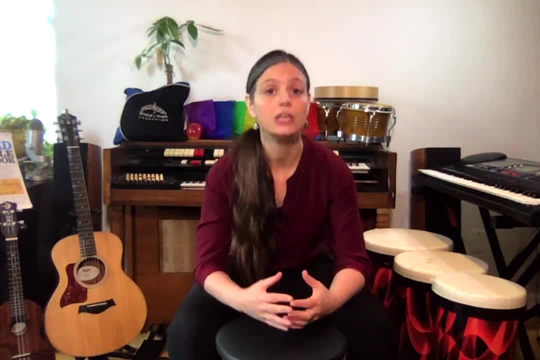 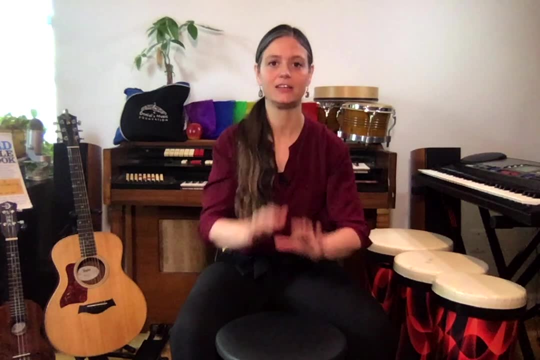 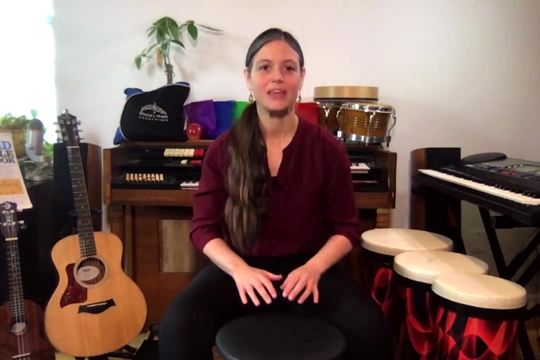 they don't like the way that feels. It's just a weird sensation. So if you don't like that sensation, you can just use your finger pads- that's the fleshy part of your finger under your fingernail- to tap. Sounds kind of like rain. Very nice, Then you're going to take. 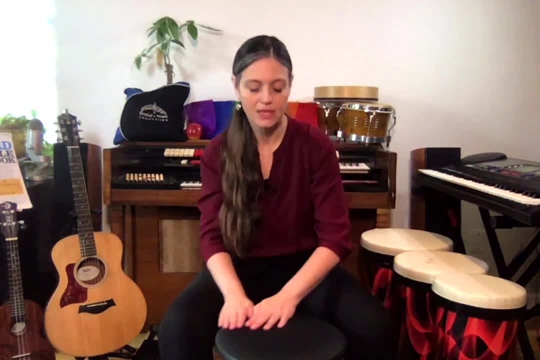 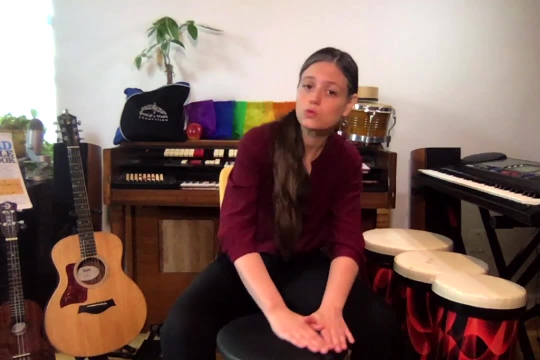 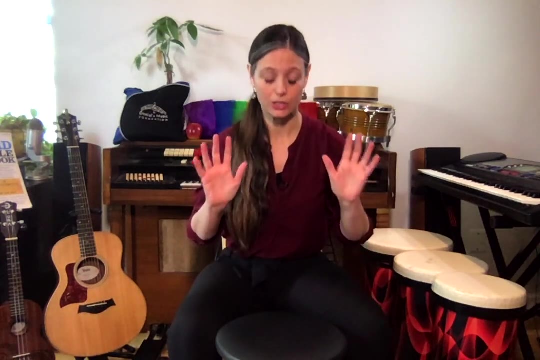 both your hands, put them palm down on the drum And push, Just push them round and round. Now push it real good, Good, And if you haven't already done this, the next part- you're going to use those finger. 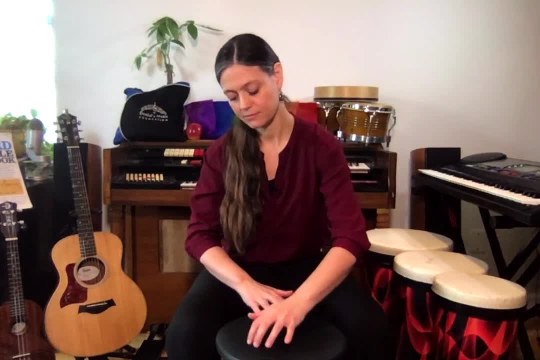 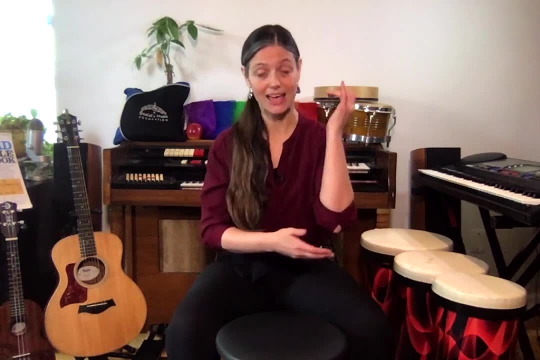 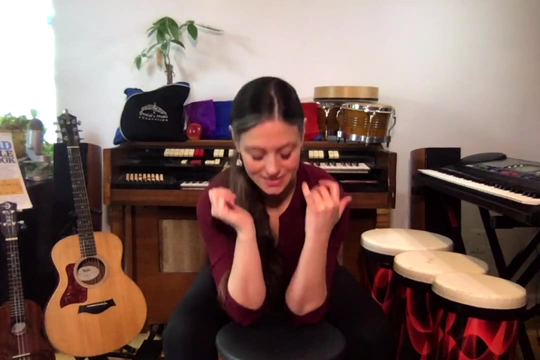 pads to tap. Very nice. Now, next, I'm going to ask you to use your elbows, if you're able, as if they're your hands. You're going to play your drum with your elbows, And if that doesn't work for you, you can. 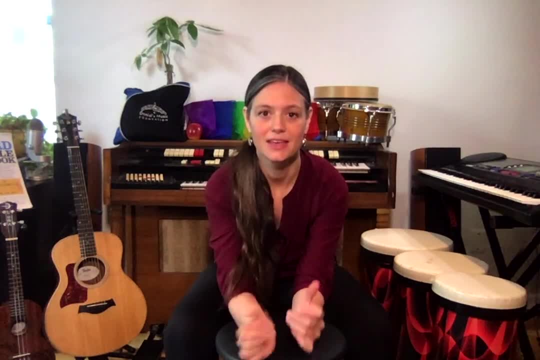 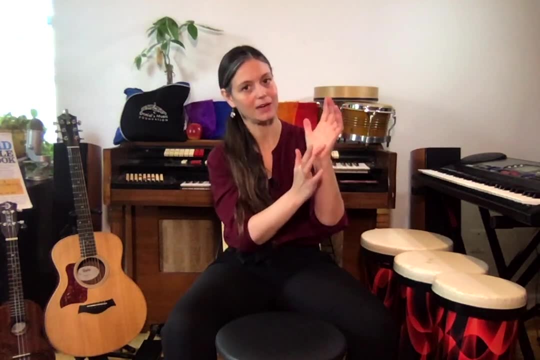 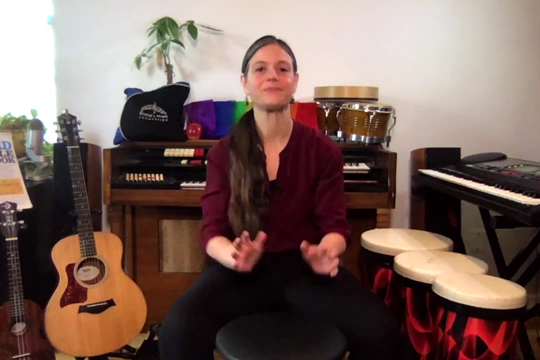 try playing with your forearms instead, And if that doesn't work for you, you can take this part of your hand, the heel of your hand, right at the bottom where your hand meets your wrist, and you can play with the heel of the hand instead. Good, Okay, The last. 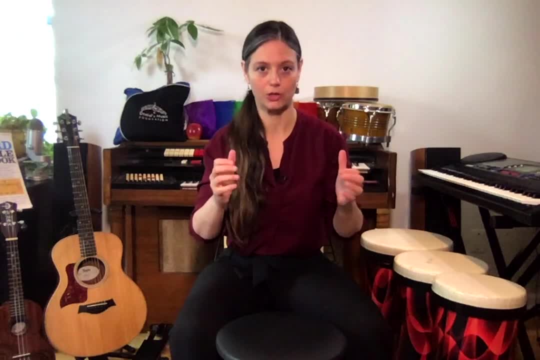 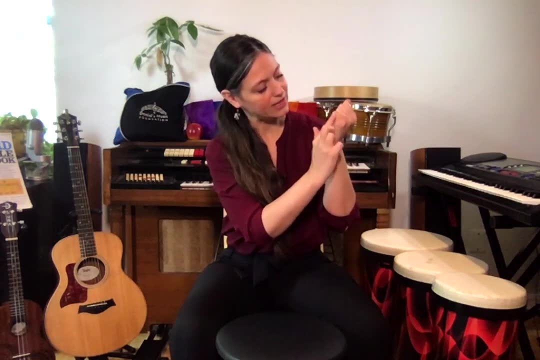 one we're going to do for that section is to pound, So I want you to curl your fingers in And then put your thumb right on top, And you're going to use the fleshy part of your hand right that's underneath your pinky or right next to your pinky, excuse me, Okay. 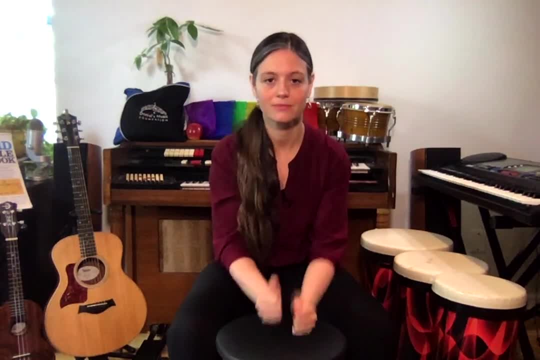 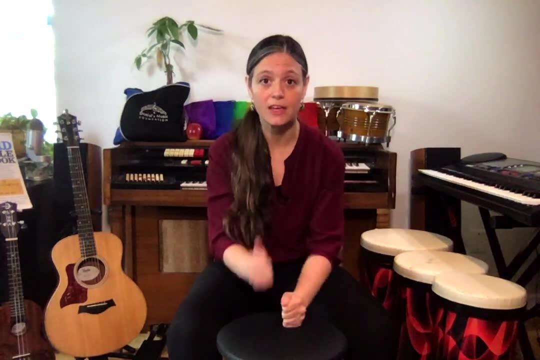 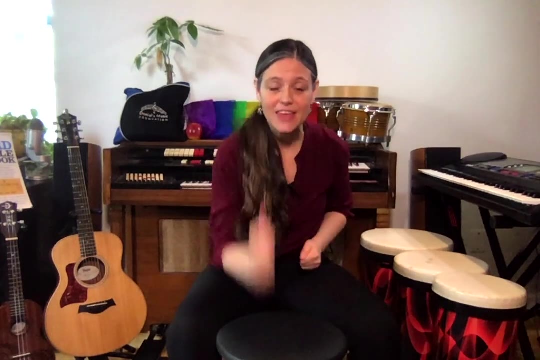 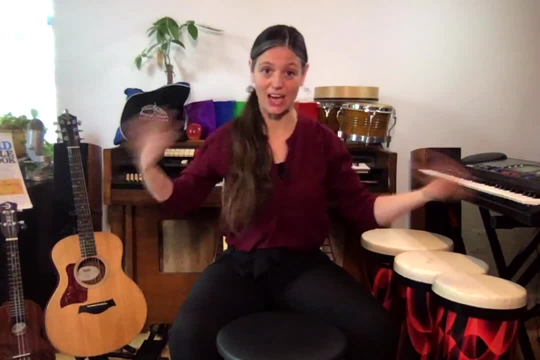 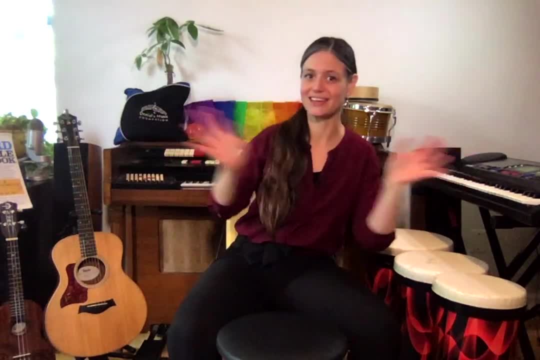 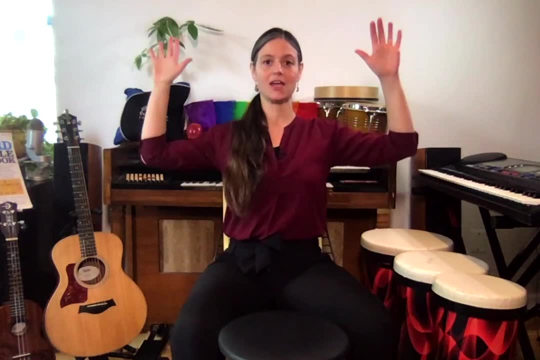 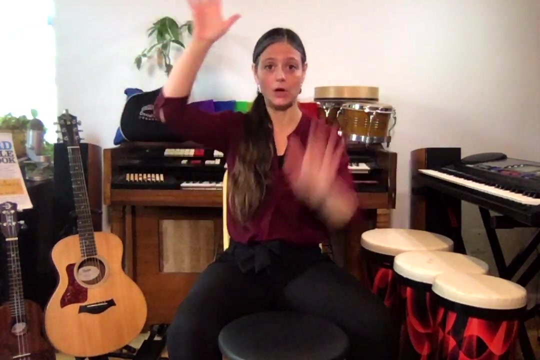 Shake, shake, shake. Shake your hands out, Shake your hands out. Wonderful, So let's go over the chorus one more time. Ready, You're going to put your hands up in the air. Bring them down twice, Bang bang, bring them up. Bang bang, bring them up. Then you walk. 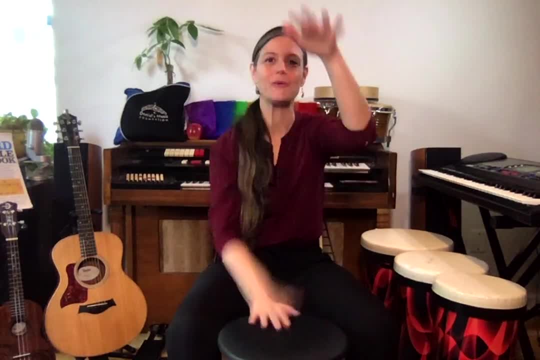 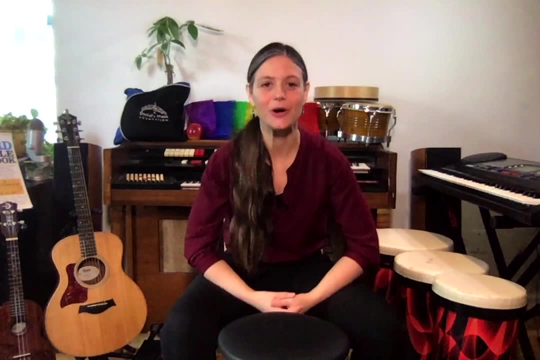 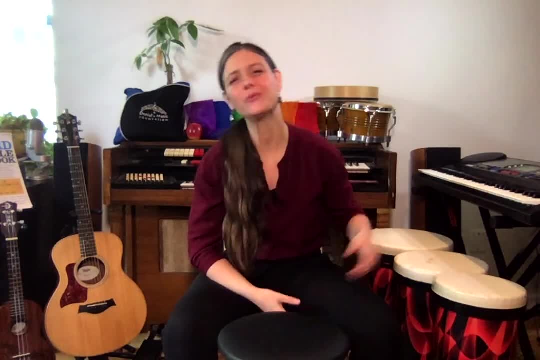 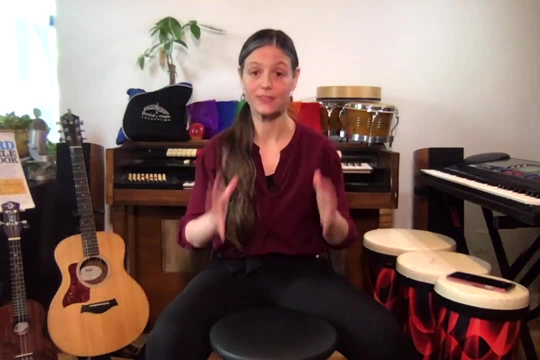 out the moves as we go, but if you miss something, don't worry about it, Just join back in when you're ready. Okay, Here we go with bang bang. Now, remember, you're going to start with the verse, so you can play anything that you want, anything you hear, anything that. 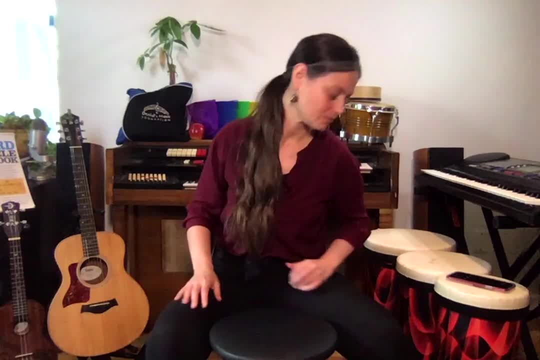 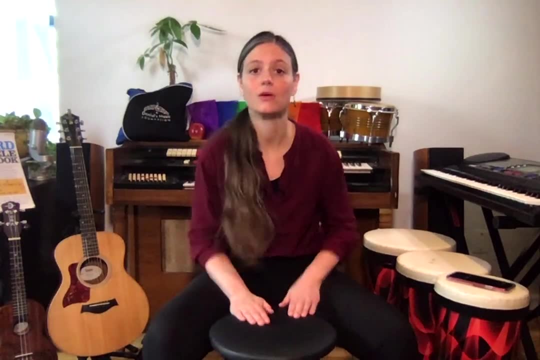 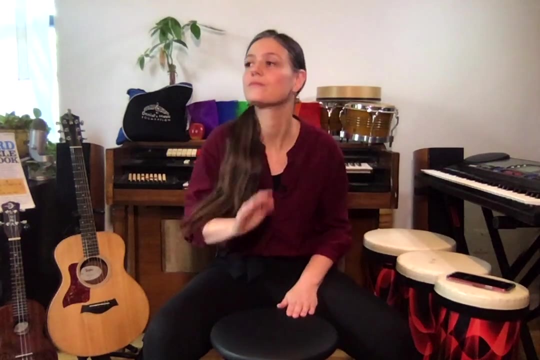 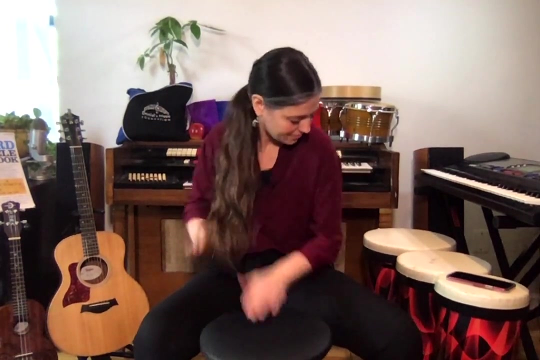 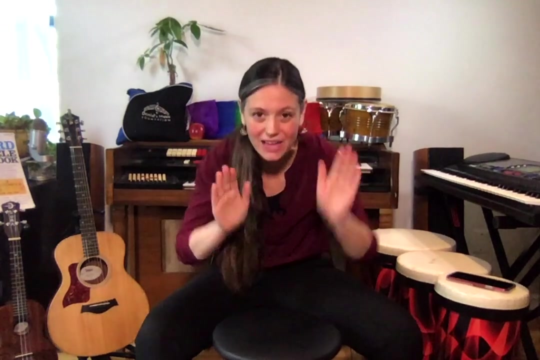 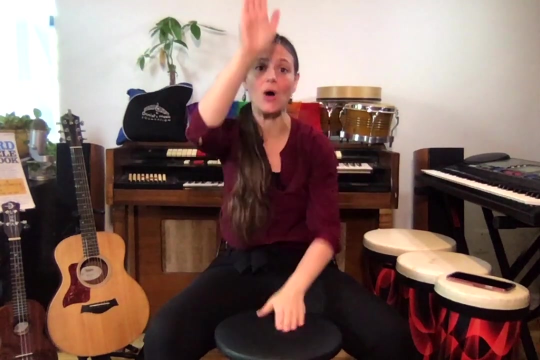 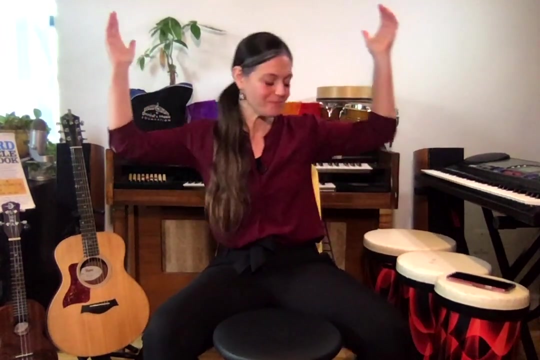 you feel Musician's choice, Okay, ready, Bang and run, and bang bang, Bang, bang up, And we walk, walk, walk, walk, walk, walk, walk, Run and bang bang up, Bang bang, bring them up, And you walk, walk, walk, walk, walk. 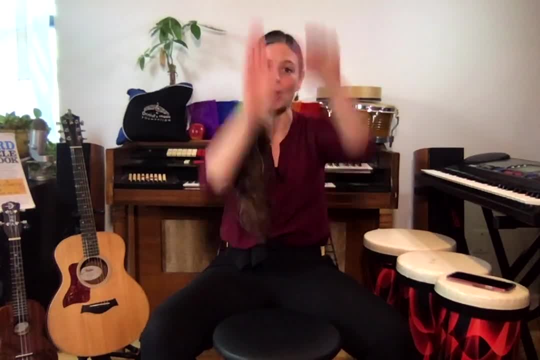 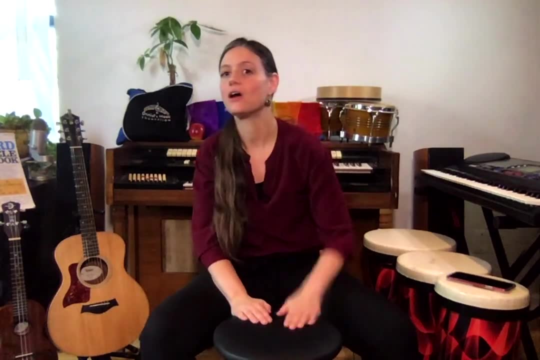 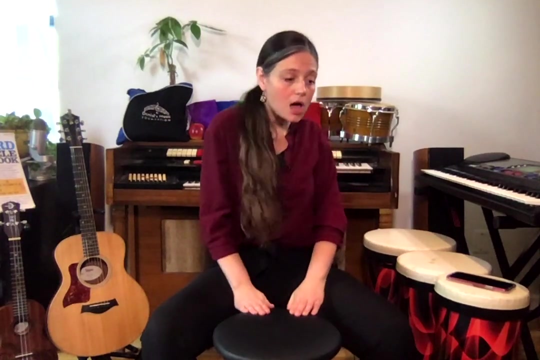 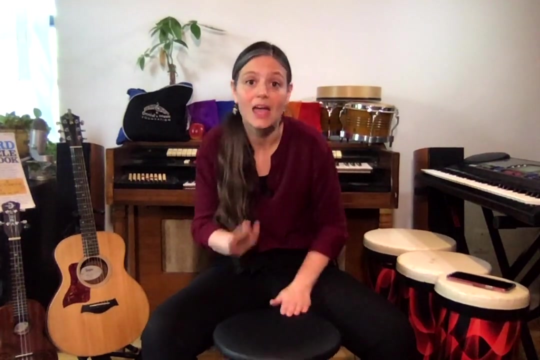 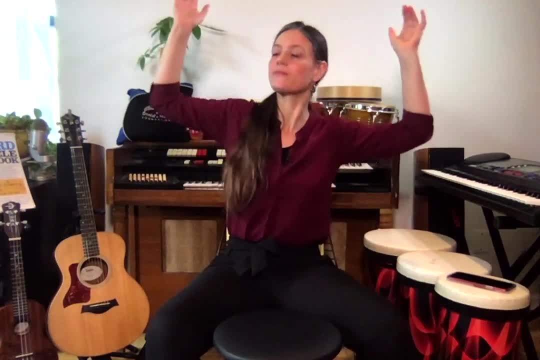 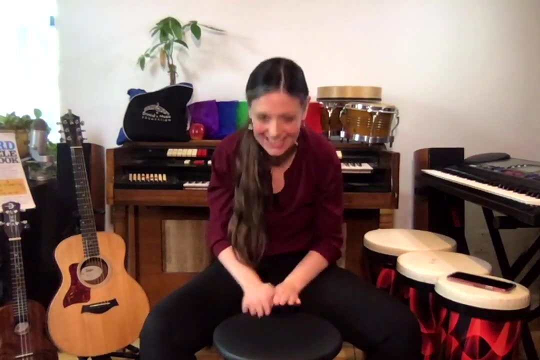 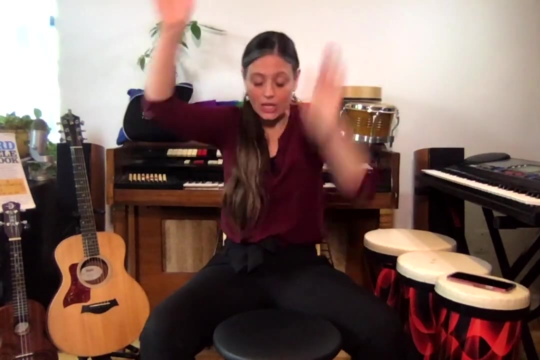 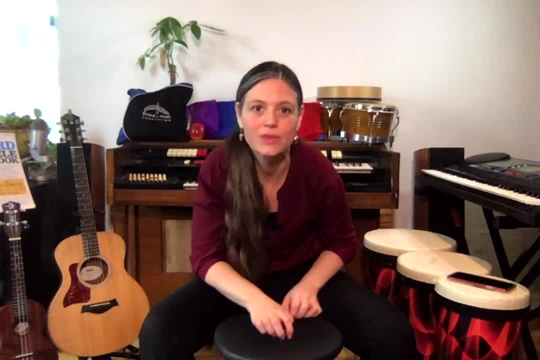 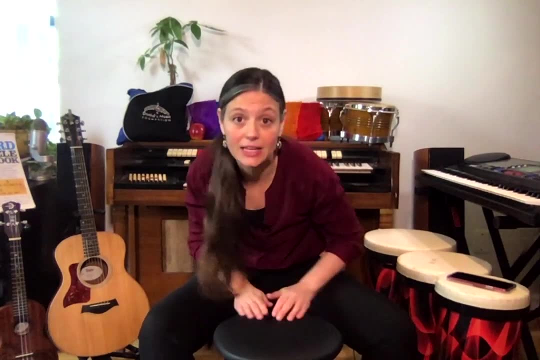 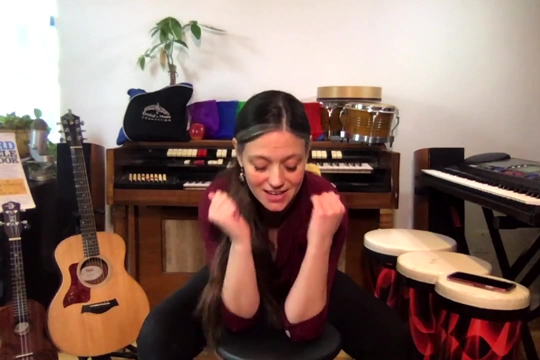 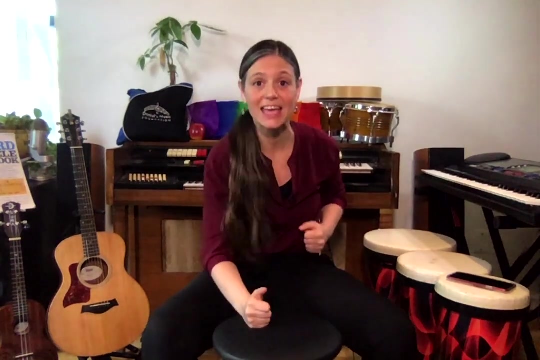 And push And push And hands out Elbows and And one, two, three, four, five, six, seven, eight, nine, 10,, 11,, 12,, 13,, 14,, 15,, 16,, 17,.